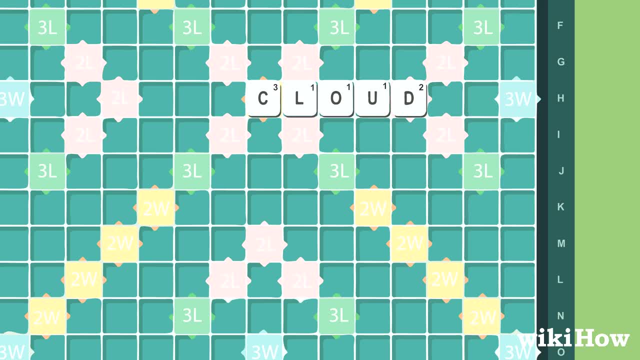 They must play a word that connects with the word that the first player made. For example, if the first player made the word cloud, the next player can use the letter D in cloud to make the word destroy. If a player makes a new word using a pre-existing word, 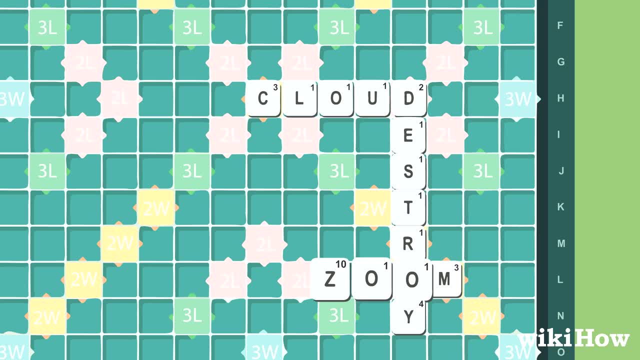 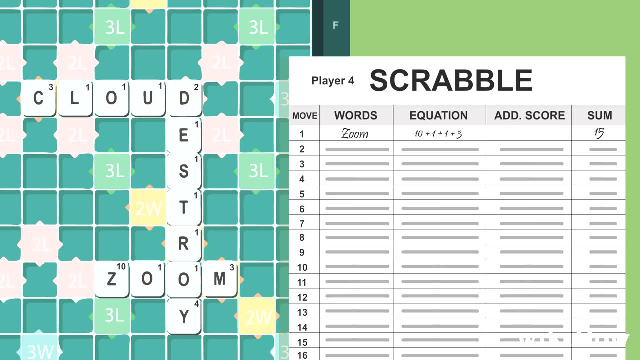 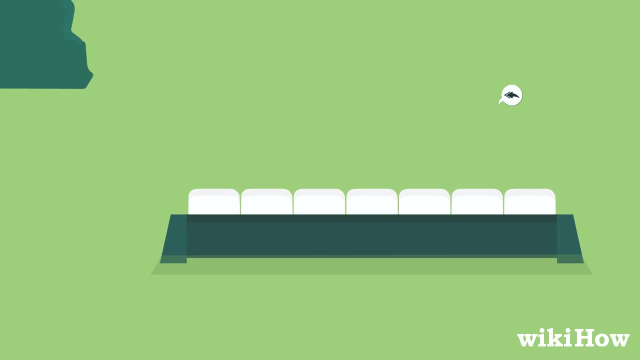 adding an M to the end of the word zoo to make the word zoom, that player adds up the total score of all the letters in that word, not just the letter they played. If a player is unhappy with the tiles in their hand, they can skip their turn and instead trade in any number of tiles. 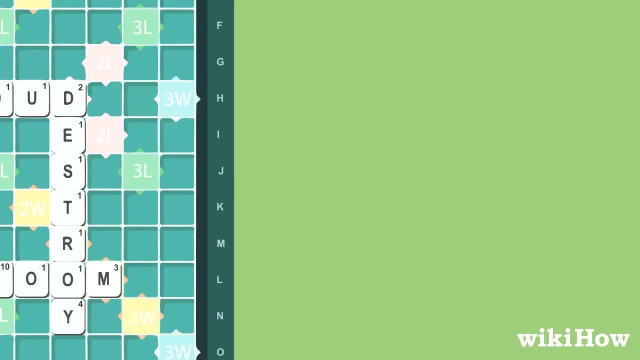 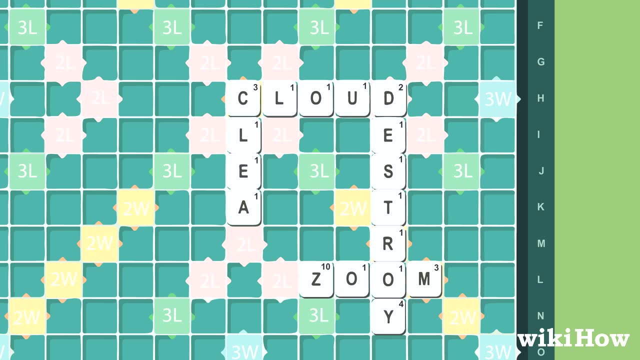 for new tiles from the bag. If a player plays a word that other players don't think is a real word, the other players can challenge it. In that case, look up the word in a dictionary. If it's not in there, it's removed from the board and the player who made it loses their next turn. The game ends. 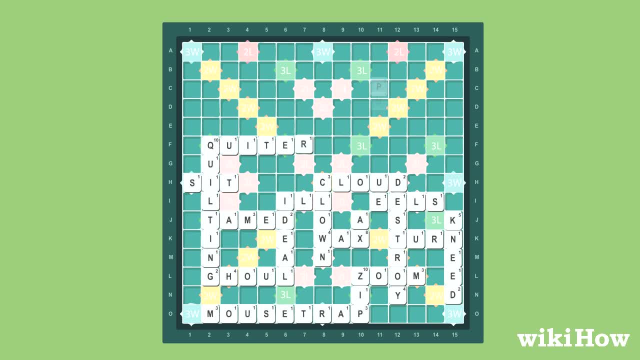 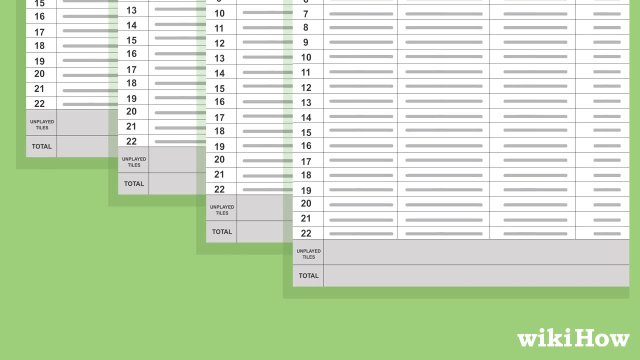 when all the tiles have been played or players can no longer make words from the tiles remaining in their hands. At the end of the game, every player subtracts the sum of their unplayed letters from their total score. After this, the player with the most points.